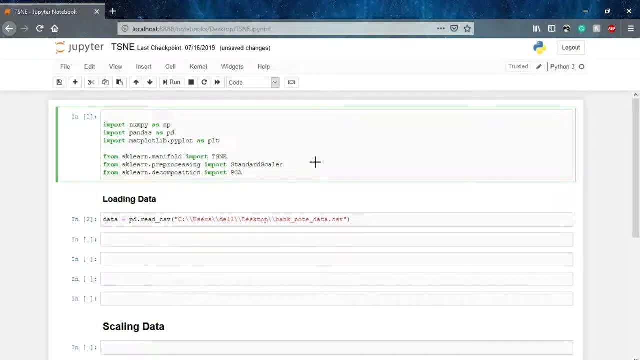 Welcome to the next lecture of the module data dimension, and in this lecture I'll be talking about TSNE. So TSNE is one more technique where you can reduce the dimensions of your data so as to visualize and get to know about the hypothesis you can use over that data or how that data is. 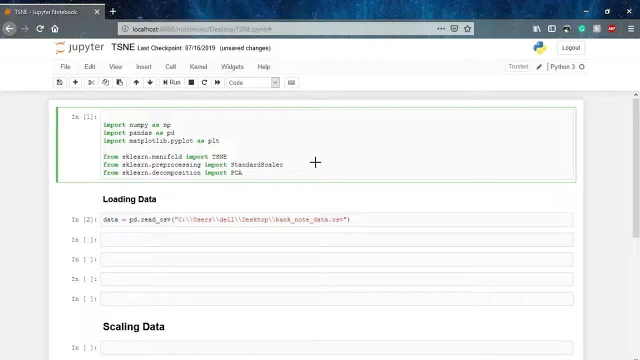 varying with respect to the parameter. So it is basically a technique to reduce your data right. So what exactly TSNE is? TSNE stands for t-distributed stochastic neighbor embedding right. It's an unsupervised non-linear technique. By non-linear I mean to say that the equation it 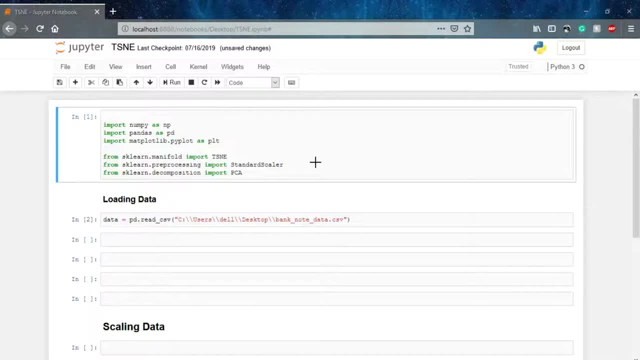 forms is non-linear, that is, you may not have a linear line when you are distributing your data. Why it is important for it to having a non-linear technique, It's because we have to visualize a different dimensions and we have to reduce that high dimensions to a lower dimensions, as per our 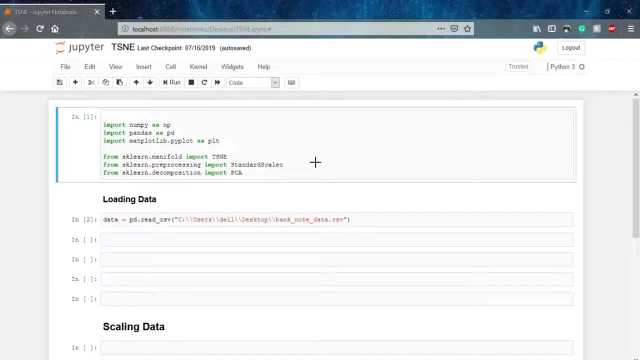 choices right. So the intuition behind the working of TSNE is that we want to see that how the data is arranged in a high dimensional space. So for having that visualization, we fit our data to a lower dimensions right. It preserves only the small pairwise distance between the data points it has. 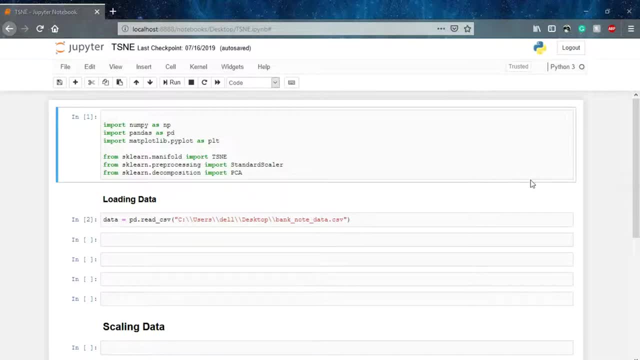 It basically calculates a similarity between the data points. It basically calculates a similarity between the data points. It basically calculates a similarity between the data points. It basically calculates a similarity measure between the pair of instances. By pair of instances I mean that if you are given some parameter- say you are given six parameters- and then you have to predict another. 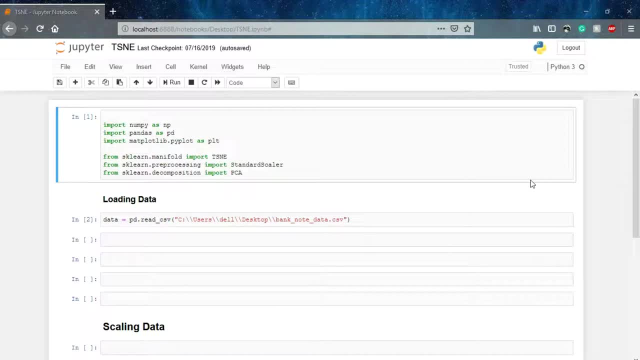 parameter right? So using that six features or that six parameter, you prepare an instance and then you find out the differences between, or the distance between, the two instances, and see that, to which pair it will belong to or what will be the final outcome for that instance. So it calculates. 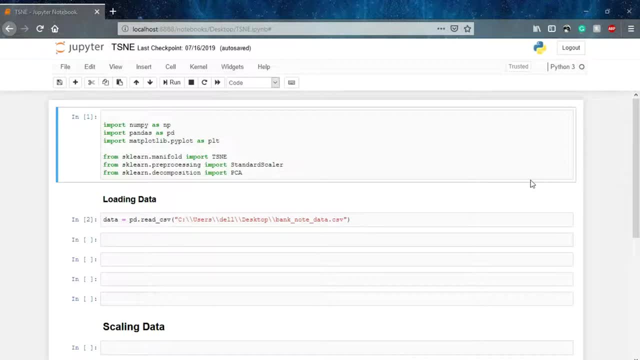 a similarity measure between a pair of instances in a high dimensional space and in the low dimensional space, and then it tries to optimize these two similarity measures using the cost functions. You don't go deep into the math behind TSNE because it's a little bit complicated For this course. you. 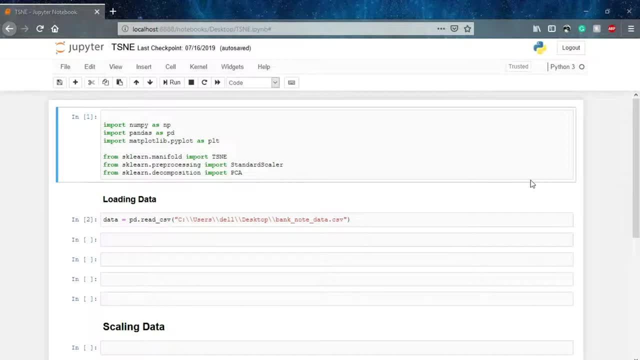 just need to understand that, how you can bring your high dimensional data to a lower dimension so as to be clear about the data you are having. So, understanding all these concepts, let's move on with our code. So I have used the libraries many fold. This is the module where you have 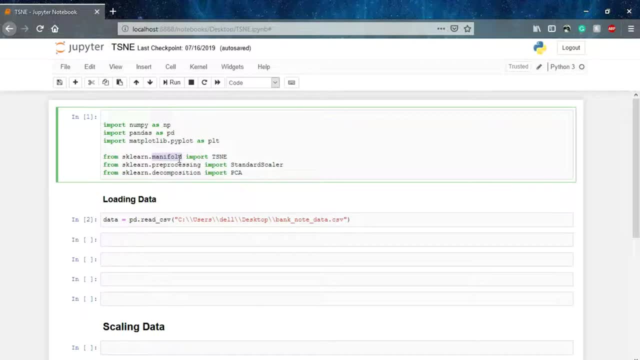 your TSNE. So I am importing TSNE from that. Again, I am telling TSNE stands for T, distributed stochastic neighbor embedding right. So I have loaded my libraries and then the data we have. So we are using a bank node data. Okay, let me show you the data. 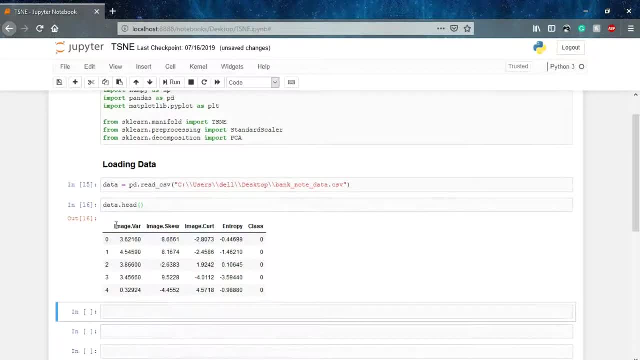 we have. So that's the, that's our data. We have four features with us and then we are predicting the class to which it belongs to, Right? So this was a kind of data where we were checking that whether this node, this bank node, is duplicate or original, one Right? So whether it's real or it's. 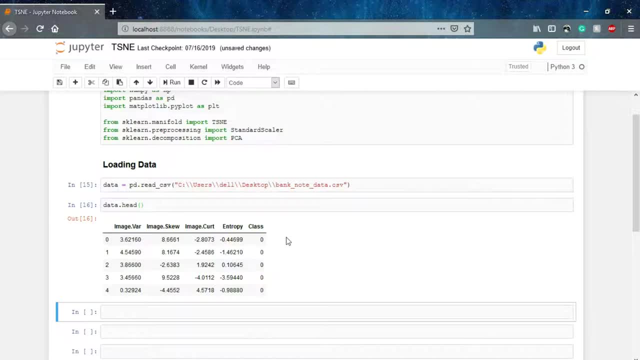 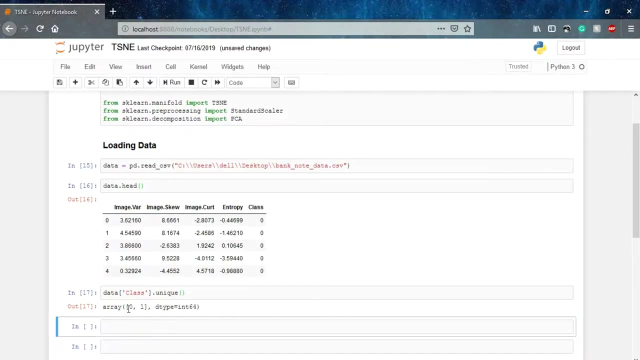 a fake money. So the class represents real or fake money. OK, So let me show you the data, The labels we have in class Column. So class dot unique. OK, So we have two labels: 0 or 1.. 0 means the fake currency and 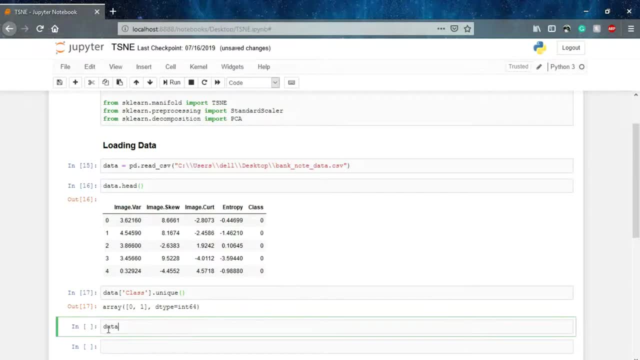 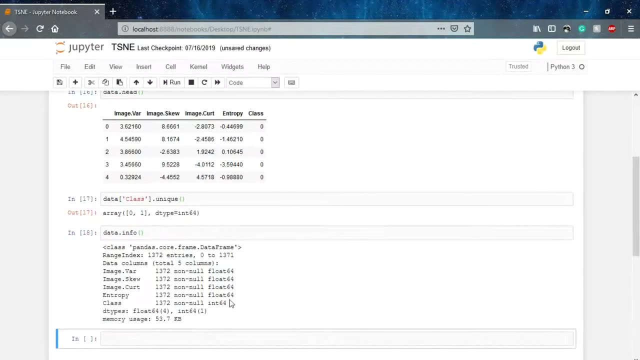 1 means the real one. OK, Let me show you the data as well. So we have around 1372 entries with us. Now what we want is we want to visualize our data, But for visualization we have to go for four dimensions. 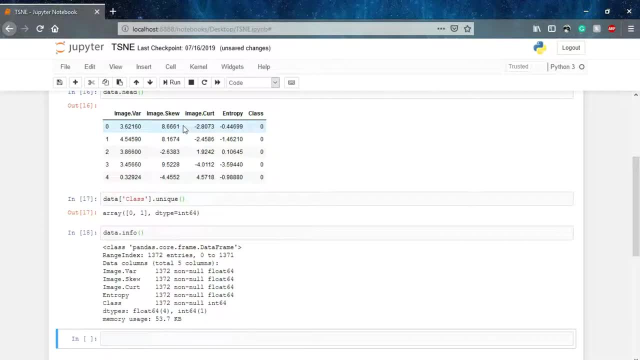 Right, But we have what? But our target is to visualize our 4D data to a two dimensional space, Right, And that two dimensional also with one dimension as the outcome, and these all input in one dimension. So we have to convert four dimensions to one dimension. For doing so, TSN works over here. 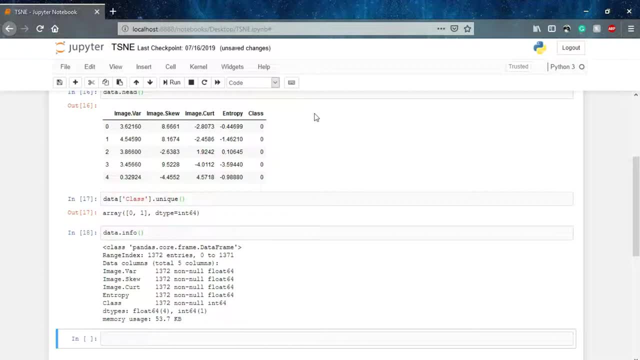 It calculates the distance, similarity measures and then between the high dimensional space and low dimensional space, And then use the cost function to plot these four dimensional intuition, These four dimensional parameters, to a single dimension Right. So this is how powerful TSN is. It makes our work. 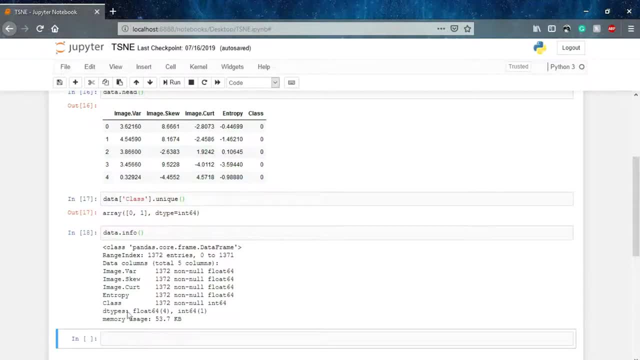 very easy. So let me show you. We'll separate out the features and the target column we have. So features we have is the image dot where. OK, Then you may use two column. Don't worry about the parameters that we have. You need not to understand the parameters, you just focus on how TSN. 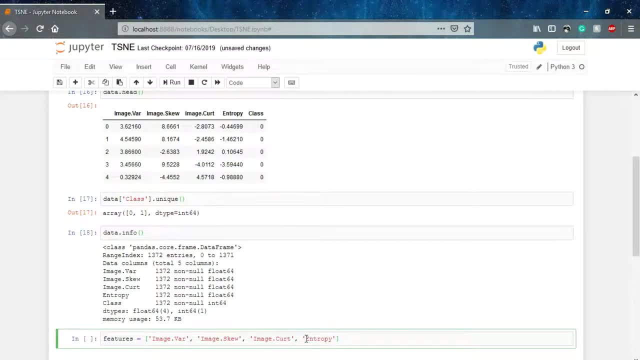 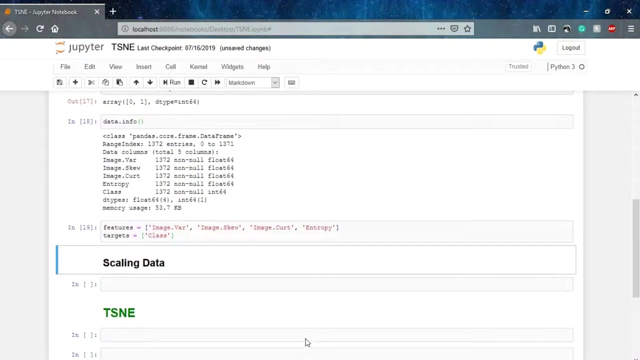 it works OK. So these are the four parameters in our input and the target output we have Is target. okay, so it's the class column right. so we have prepared. now what we have to do is we have to scale our data, because the data dimensions we have, or 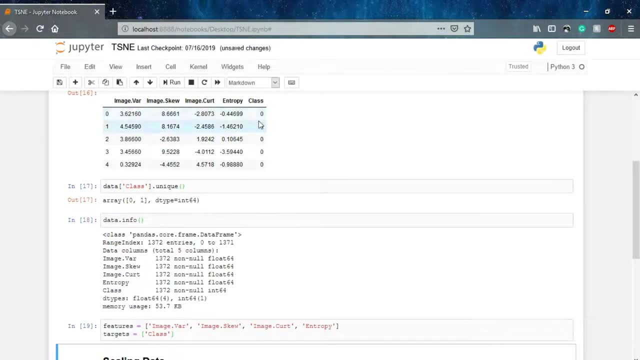 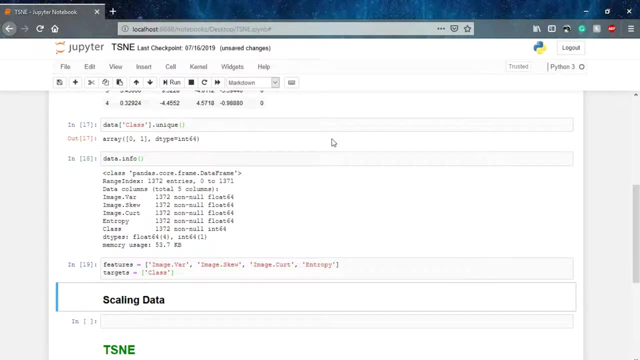 the range of the values in each parameter is different. so to, as I have explained before, to make our model unbiased, we have to scale our data for a uniform distribution. okay, so what we'll do is let me know data norm, that is normalized data, so we'll copy our data to it because we'll keep with us the 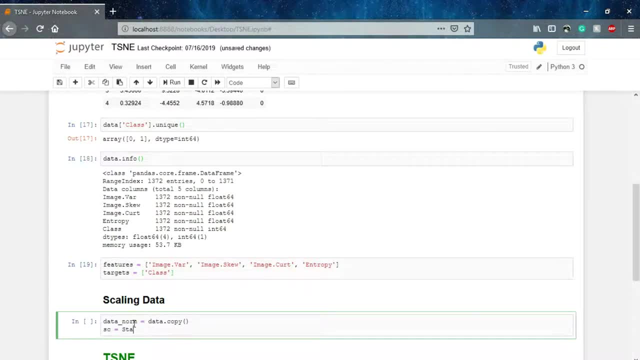 original data as well. so we will say: now we initialize the standard scalar, we have so standard scalar, okay. and then what we have to do is we have to fit our data to the standard scalar and we have to transform our data so data norm and we have to play with the features only so data norm features. 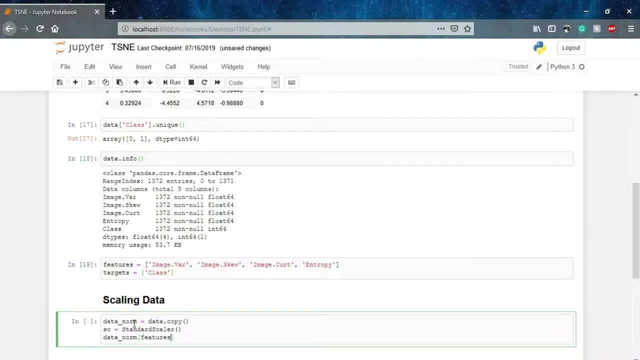 features right equals to standard scalar dot fit. what we have to fit is we have to fit the data, that is, the data features, the original data. we will take the features only so features, and then we have to transform it also, so we can do it along with this part, so also transform it and then transform, but and 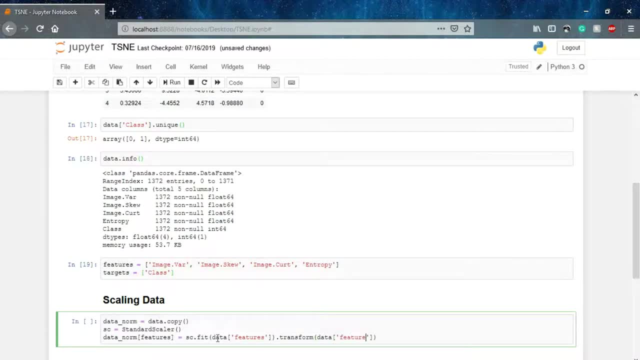 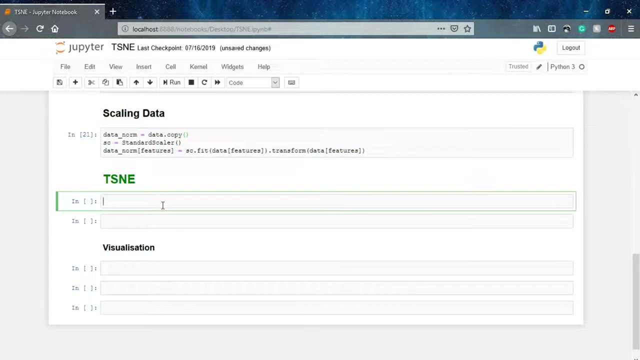 transfer data features. so first we have fitted our data over the data features, then we have transformed the data, and the transform data will then go to the data norm features. okay, now what we have to do is we have to plot our today. so for that we have to initialize the ds and he model. it's a 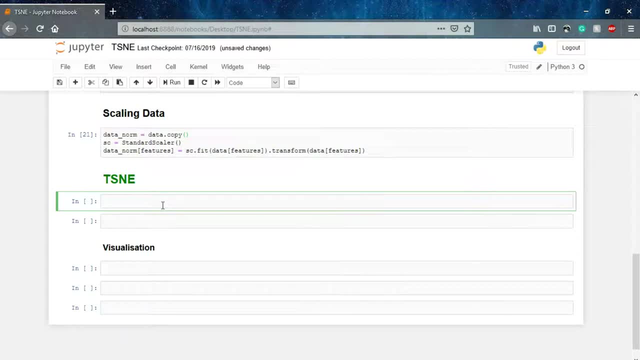 supervised learning model. so we have to initialize it, so let's name it at PS any only so PSM equals to initializing the t SnE model that we have loaded above- then have to set the learning rate, as we are doing in our machine learning models. you can take example. 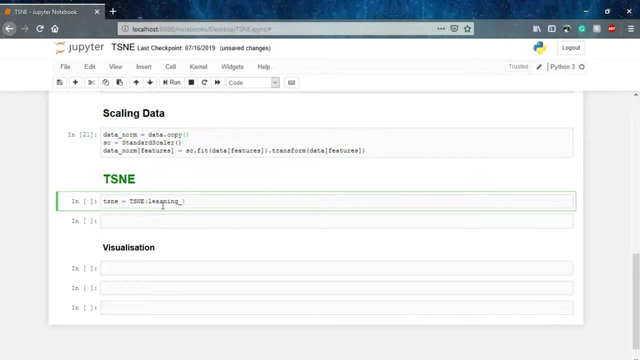 of linear regression, as in that case we have also used a learning rate. so in this case, let's set our learning rate to be 500. okay, and the number of components we want? so i want two-dimensional, i want to convert my data to a two-dimensional space. so, number of components i want: i want two. 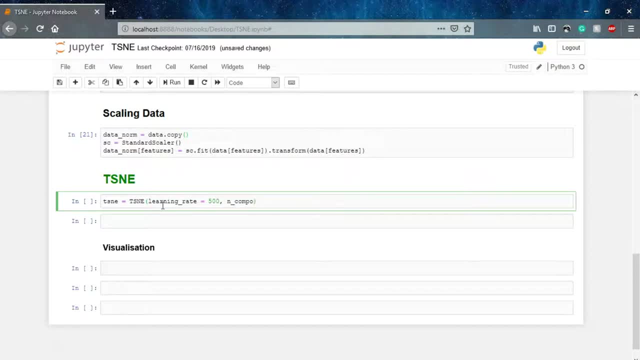 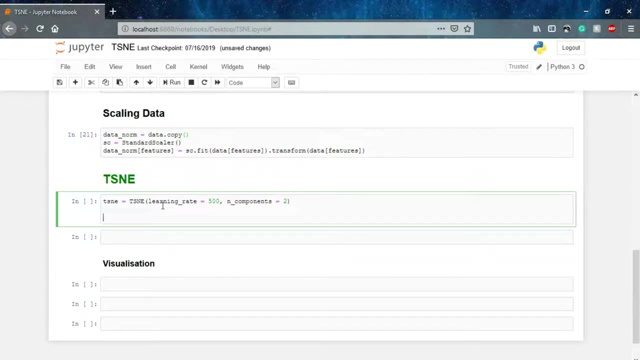 components. so number of components: components equals to two. okay, and then we have to transform our data. so let's name the data as xtne, because that's the feature data we have. so xtne and tsn dot fit transform. now we have to fit transform our. 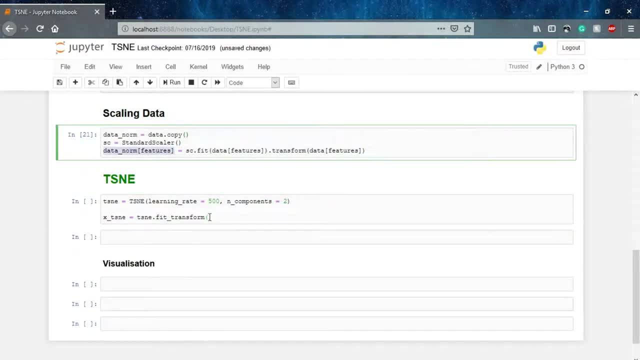 data into the data norm features: right, this will be the input. so that's why xtne and similarly, we'll prepare the ytsne. that is the output. so ytsne equals to data and the normal targets that we have to predict. so the output column data targets. right, so it will take some time. yeah, it's ready. 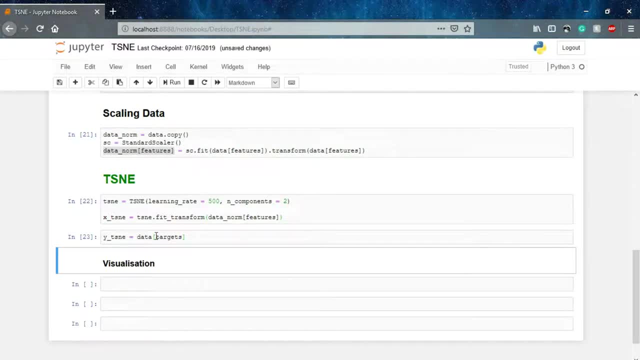 now. so we have our input xtne and the output is ytsne. so xtsne is now being converted to a single uh, a uniform data. and when we basically this data norm features was the scale data. it has all the four parameters but those were scaled. now, when we fit transform our data using tsne, it has converted that four. 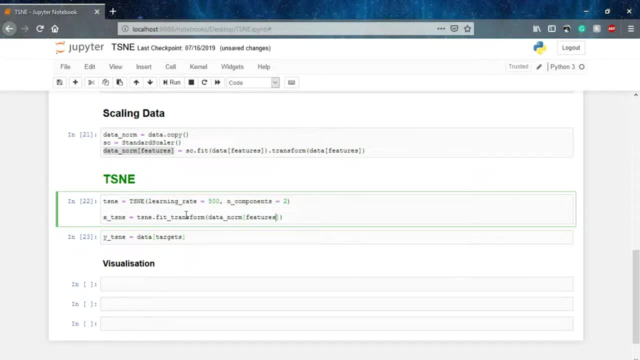 dimensional data to a single dimension, and now we have two dimensions with us, that is, x data and y data, and we'll be plotting an xy correlation to see the two-dimensional plotting of our data. okay, so this is how easy it is. so for visualization we will use matprolib. so plt dot figure. let me set the size. 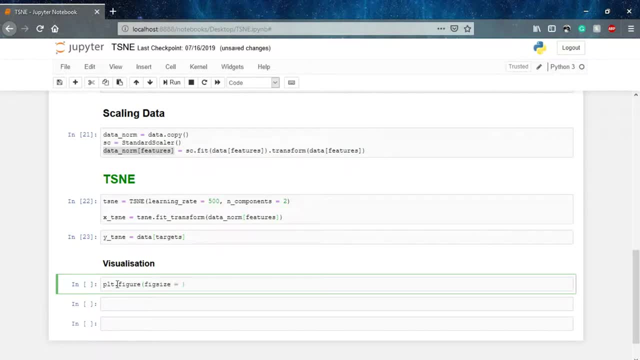 of the figure. so figure size equals to, let's say, 16 by 11. okay, and then plt, dot scatter, and what we have to plot is we have to plot xts any and the yts any. so we'll say xts any and mp dot where? 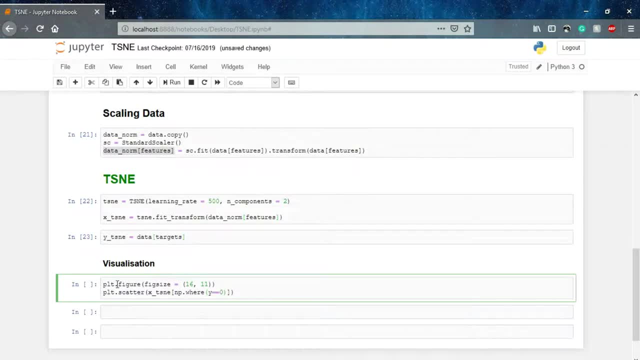 y equal equal to zero. plotting it with the zero, okay, and then x, so we'll say x, tsn, e and p dot, where y equal, equal to zero with respect to one, and okay, sorry, right. and then color equals to green. let's set the marker also. so marker b: 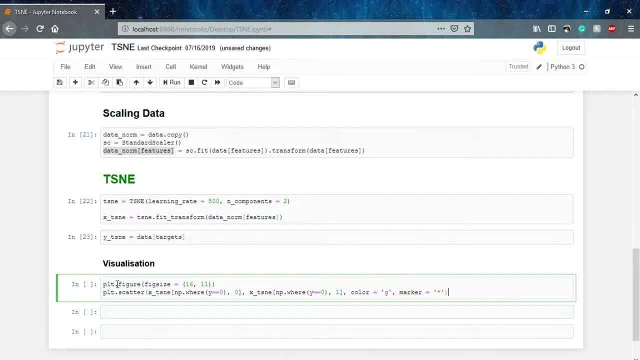 star. okay, so marker b star and again copying this: okay, so xtn e where this y value equals to one with respect to zero, and where y value is equals to one plotted with one. okay, so let me just explain you what, what we are doing over here. 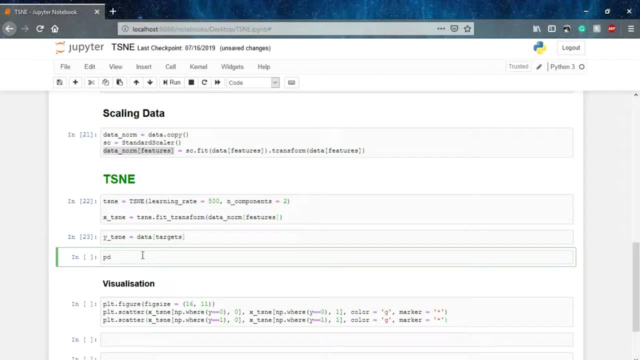 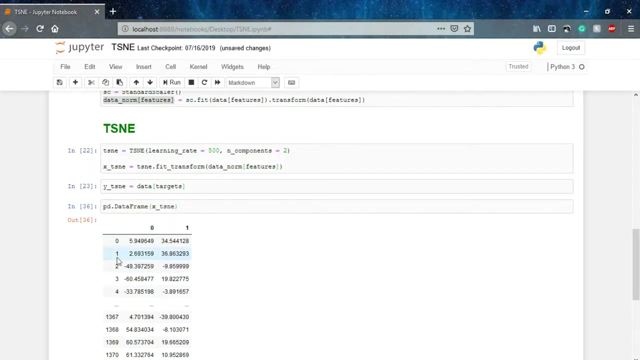 so initially we were having the xts any. so pd dot. let's say, let me show you pd dot data frame. so what data we are talking about? we are talking about xts, right? so xts any. so this data was having zero and one dimensions, right? so these are the two dimension and these were rest of the total entries. 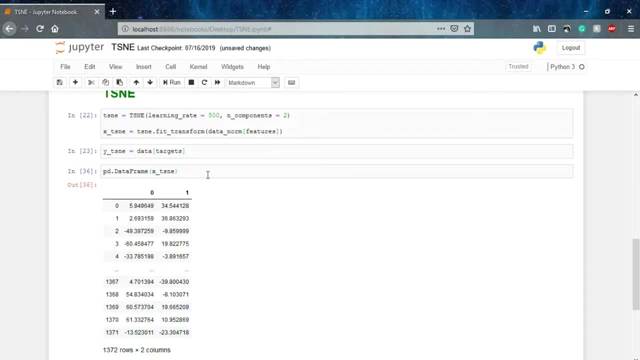 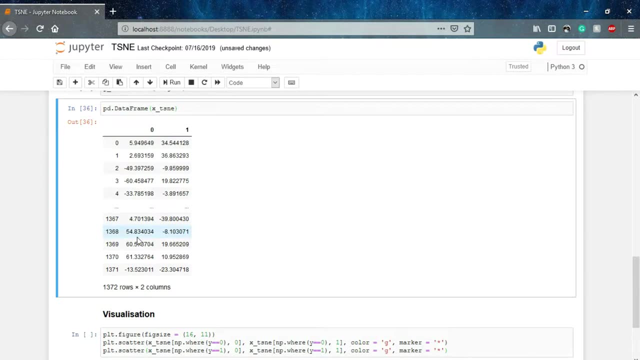 we have right. so 172 entries, two columns. now what we are doing is we are basically plotting the data, all the all the data: 0 with respect to 0, 1 with respect to 1, 0 with respect to 1 and then 1 with respect to 1. so that's what we are doing. 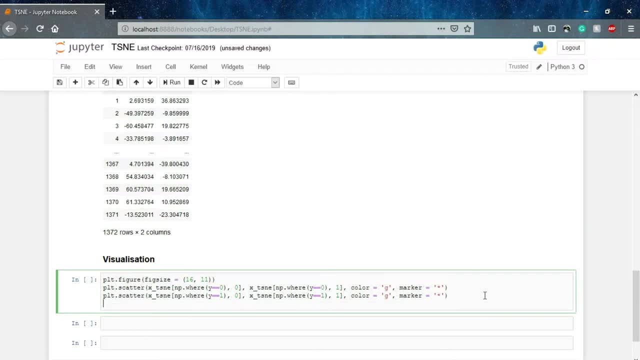 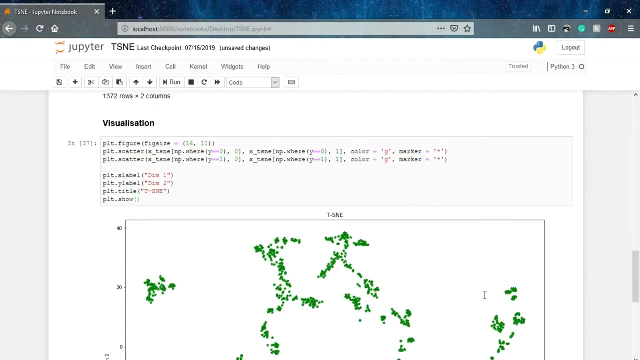 over here. that's how we are scattering our data. also, if we say, let's say plt dot, x label and set the data dimension as dimension 1 and then y label as dimension 2, okay, and then let's title it as the ds any graph, so t s any. now plt dot show okay. so now you can see. 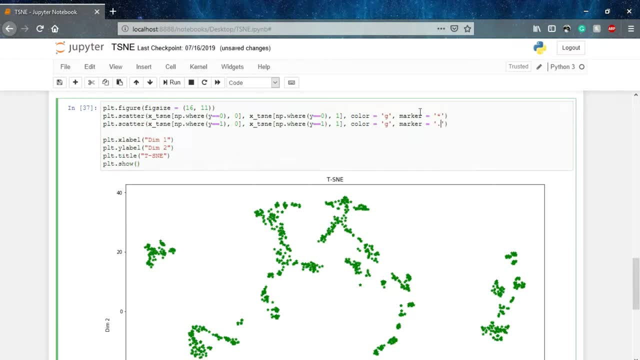 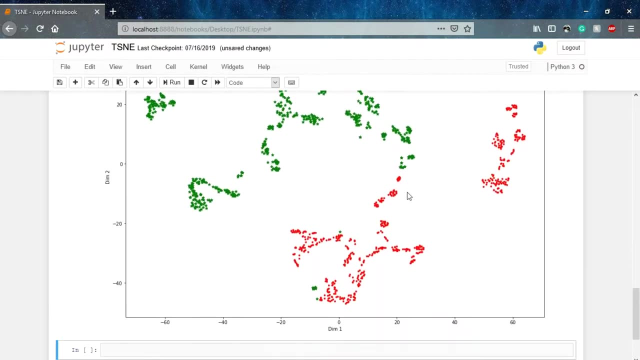 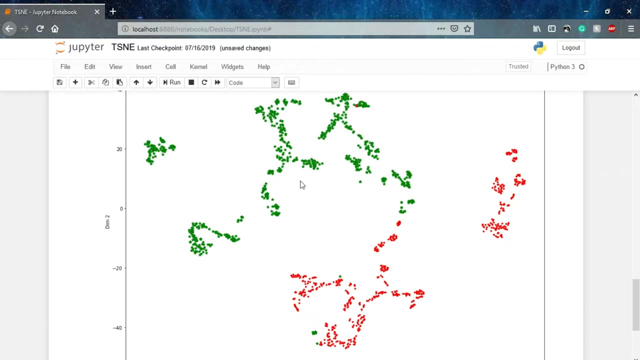 okay, i have. i have done a mistake. the markers are same and curves are same. let's change it. okay, so now you can see. that's the graph we are finding out from this data. so we have basically converted a four-dimensional data to a two-dimensional data. we are plotting our 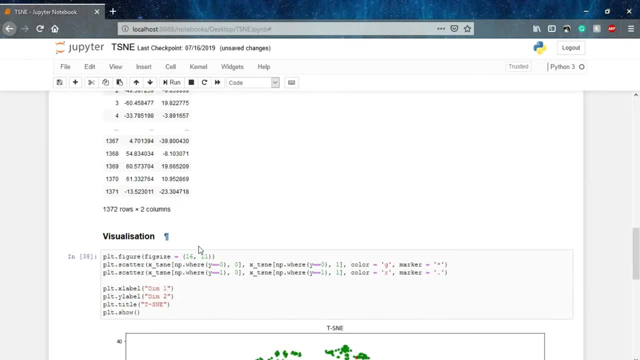 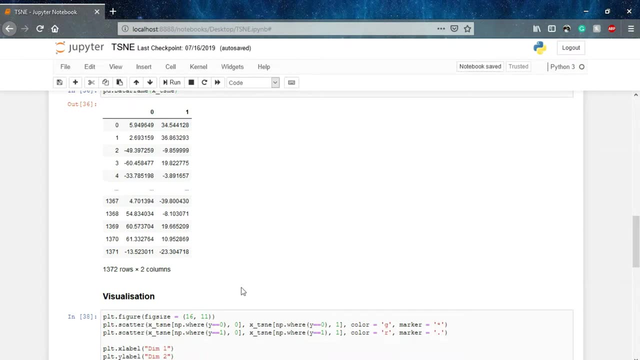 data x, t s, any with respect to y, and it's taking each column with respect to the class of y each time. okay, so what we are doing is we are plotting x, t s, any data where y equals to 0 and the data is 0, and. 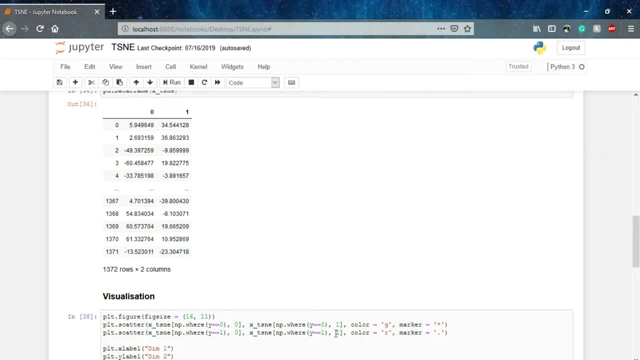 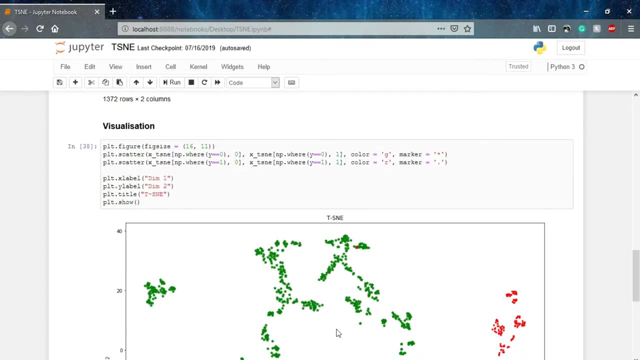 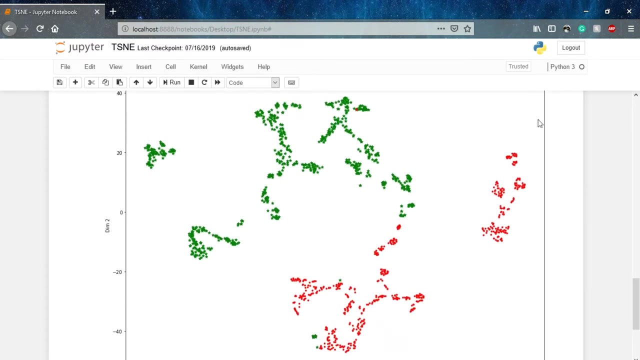 similarly, where the data was 0 and the label was 1. so we are doing all the pairing and then scattering using the scattered graph. we are plotting that data over here. so now you can see that this is the data we have. this is how we can visualize our data. you can see that in high. 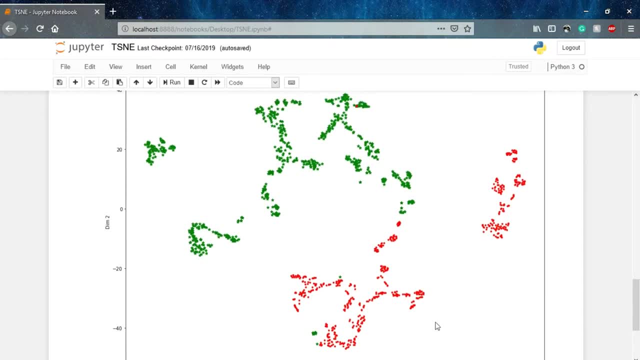 dimensional space are. our data can be easily be separated out using any hypothesis. if we are using a linear hypothesis, you can- you can think about it as in a high dimensional space. it's just an intuition for you to visualize how your data is plotted and how your hypothesis can work, for example, if you will be having a red. 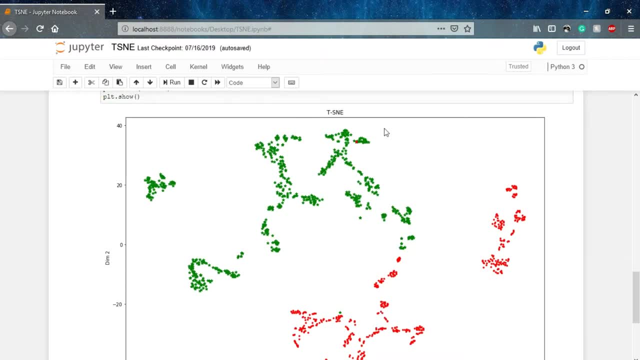 uh, these red marks over here also. then, in that case, to separate out this green data, you have to use a ellipse, so you can have an idea of how your hypothesis work and how your model can be used for such kind of data. okay, so this is how we use dsne. this was all for this lecture. this is how we convert a high